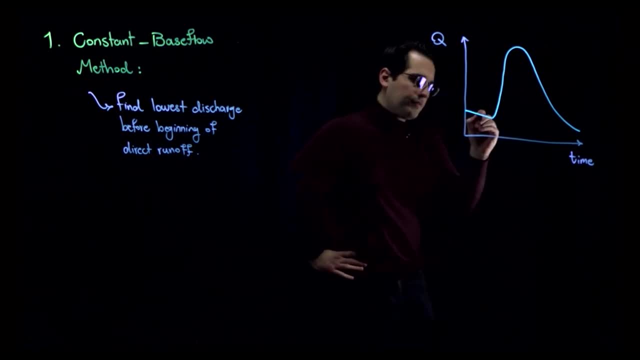 beginning of direct runoff. you're going to tell me that the beginning of the direct runoff is going to be this point. Why? Because right after that, hydrograph starts rising. So this would be the rising limb of the hydrograph right. So to find the flow of that point, I just need to find the flow over here and I'm going to call it q. 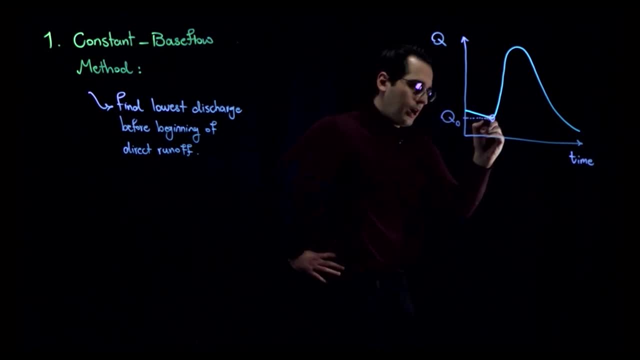 sub zero, And the corresponding time for that would be t sub zero. As its name suggests, the base flow is going to be constant, right? So you are going to add a horizontal line until it intersects the falling limb of the hydrograph. in this point, This point time, let's call it t1, and flow is going to 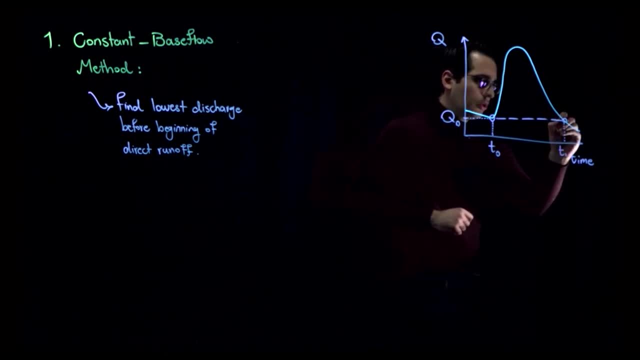 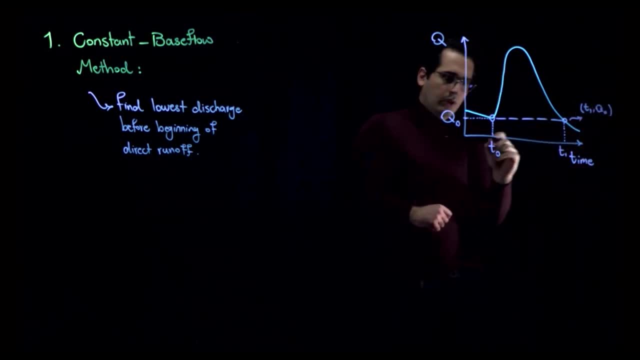 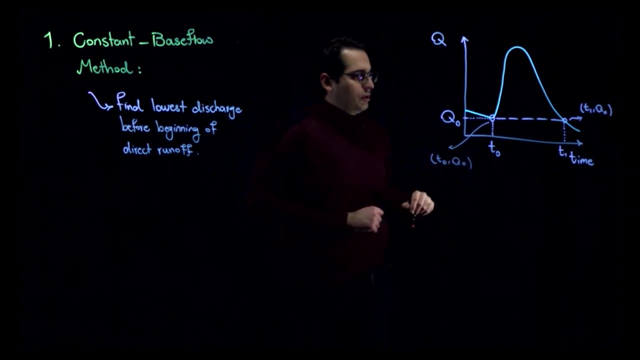 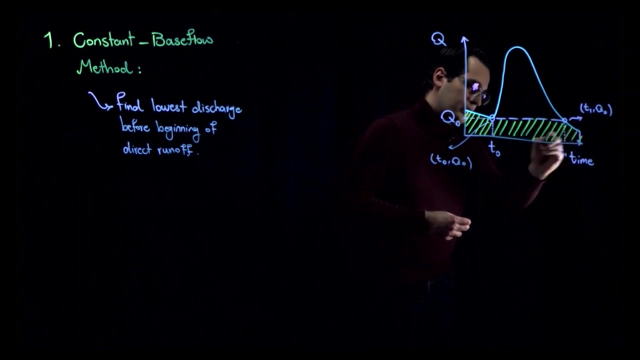 t1, q sub zero, and the ordinance of this point, t sub zero, q sub zero, Perfect. So now, whatever is below this constant line that I'm going to show it to you, whatever is below this constant line, this is your base flow, according to constant base flow method, And above this line is going to be your. 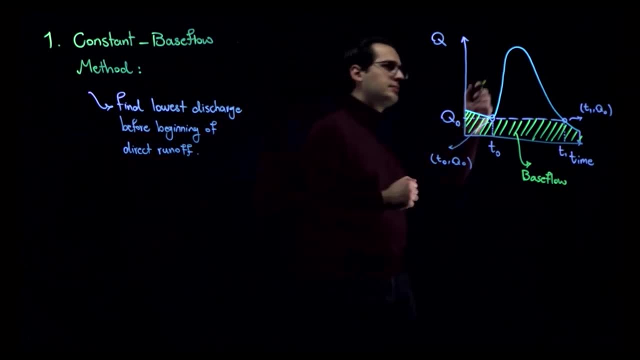 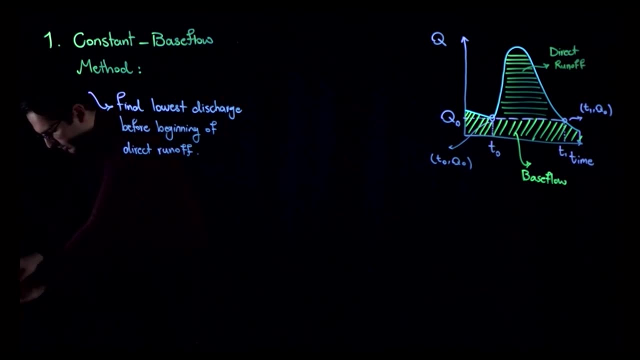 direct runoff. So now what I'm going to do is to write an equation that describes this process that I showed you over here. Notice that what we're going to find is qb at time t. qb at time t represents base flow at time t. 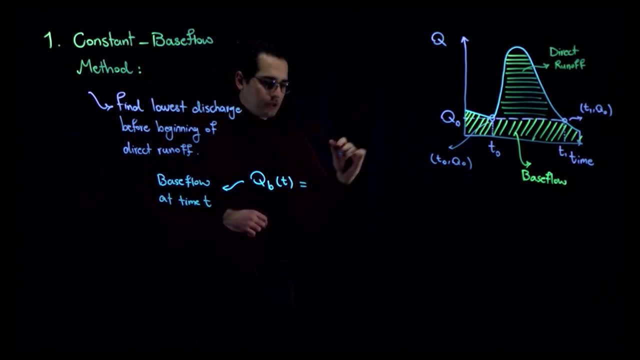 Alright, so I'm going to write a set of equations that describe what I told you over here. There are two different times- t sub zero and t sub one, So I'm going to define the base flow based on these times. So if 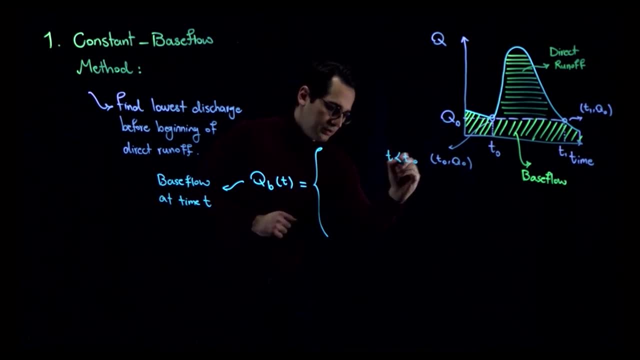 time is than t sub zero, if time is in between t sub zero and t one, and if t is larger than t one. okay, so if t is less than t sub zero- we're talking about this section right. as you can see- the base flow is going to be equal to the value of the hydrograph. what is the value of hydrograph? 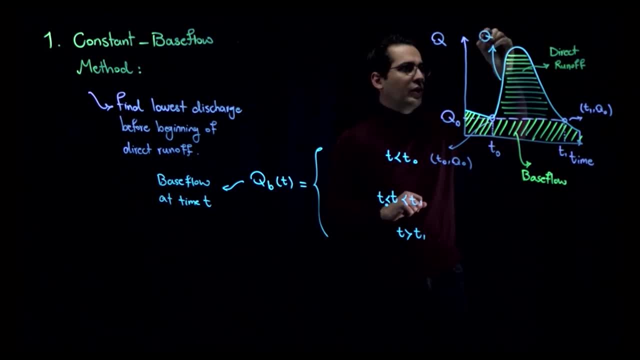 this blue line right. the blue line would be q flow at time t. so before the beginning of the direct runoff, the value of base flow is going to be equal to the value of hydrograph at time t, when time is in between t sub 0 and t sub 1. over here you can see that we have a constant line. 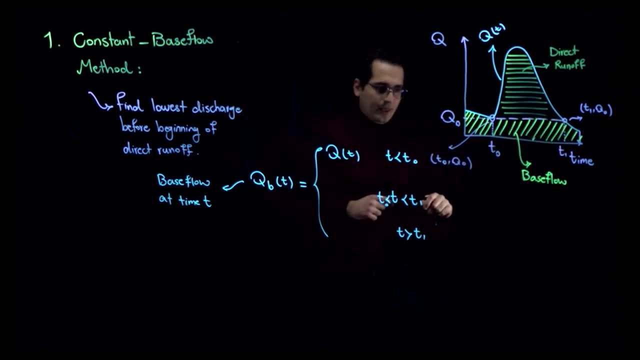 right, it's a constant base flow method. so base flow is going to be equal to the constant value of q sub 0. that's a constant value, right. and then, after t sub 1, over here again, base flow is going to be equal to the value of hydrograph, or q sub t. this is the equation that we are going to use. 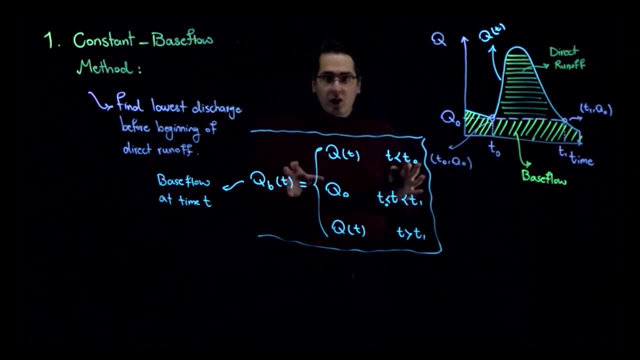 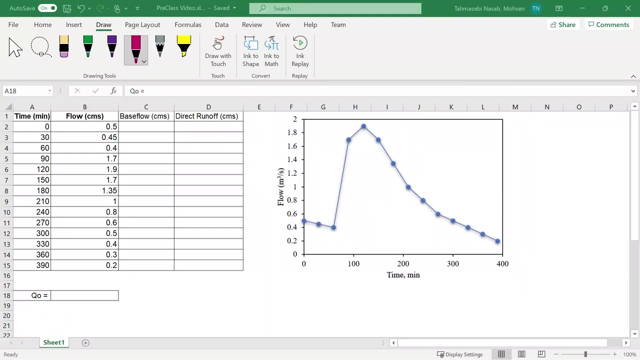 in our spreadsheet in excel to be able to automate this process and figure out the base flow for any given hydrograph that we have all right. after this, i'm going to show you how to use this equation in an excel spreadsheet to separate base flow from direct runoff. so i have a hydrograph. 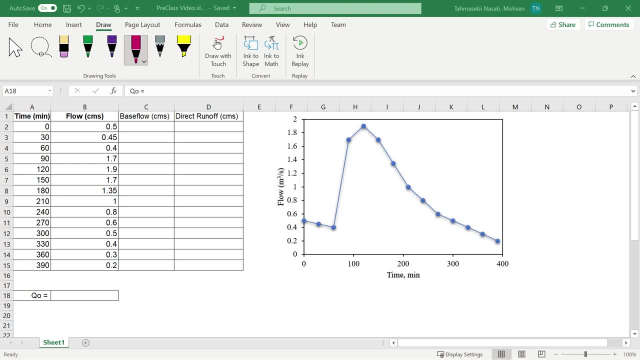 time versus flow, and i want to find base flow and direct runoff. the first thing that i need to do is to figure out the value of q sub 0.. this q sub 0 is the flow of hydrograph when direct runoff starts. so right over here i know that this value is equal to. 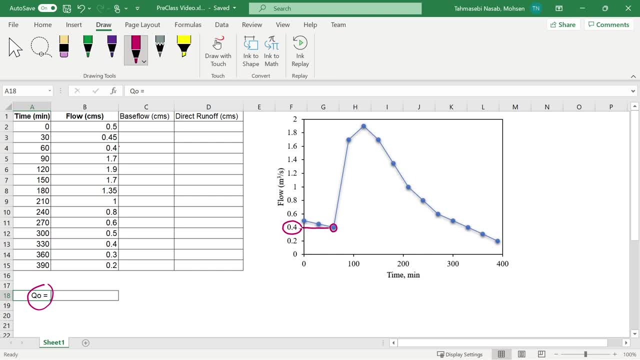 0.4. so from the beginning of the hydrograph, this is the value that i'm looking for and this is the time that it starts. so this time is 60 minutes. whatever i have before, that is going to be my base flow. so before that, this line represents my base flow. whatever is under that line from this: 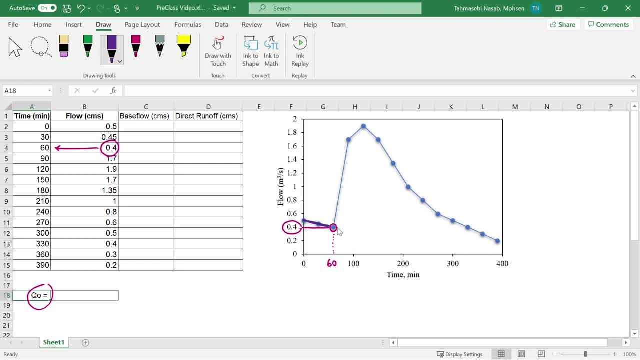 specific point. i am going to draw a straight line because it's a constant method. this represents my base flow all the way to this point, because the flow is 0.4 and time is 330.. and after that point, this line represents my base flow. so the area below this perpendicular line, 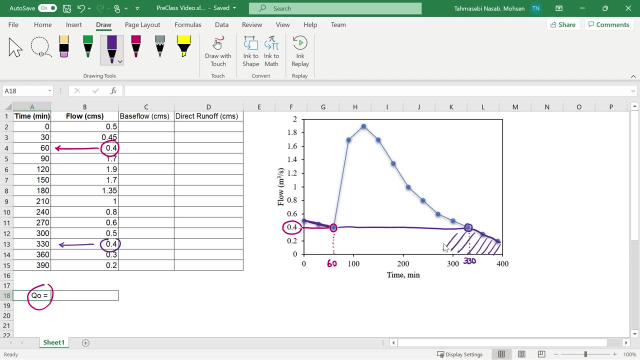 the area that i am shading right now is the base flow for this hydrograph. this is base flow, but how do we show that in excel? okay, so the first thing that you need to do, you need to define your q sub 0, and i'm going to define that 0.4, as i showed you on the graph. all right? 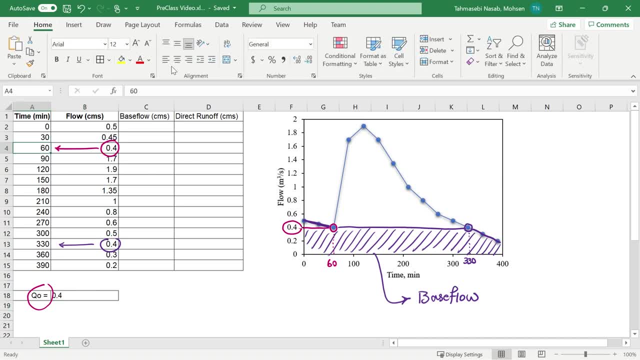 before this point, before this specific point, and let me, there we go before this point, whatever base flow that you have is equal to the flow of the hydrograph, to the value of the total hydrograph, right, okay, so this is going to be, for example, equal to the flow of the hydrograph. next it's: 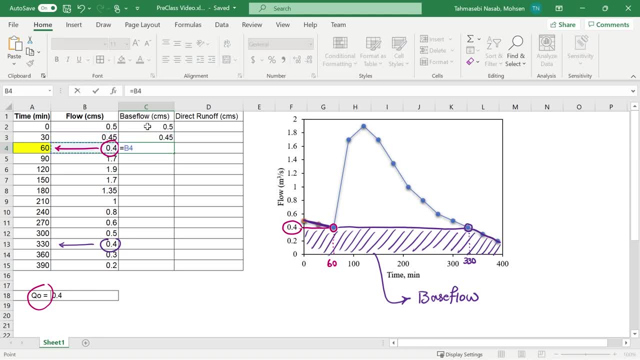 going to be to the equal to the flow of hydrograph. next is going to be equal to the flow of hydrograph. okay, and take a look at right now. you can see that the hydrograph is of the base flow is represented on the hydrograph too. let me just for the purpose of making it clear, 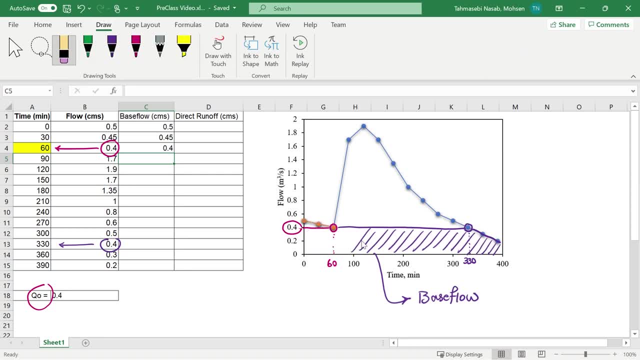 let me just remove this, what i have over here, so you can see what's going on. all right? so after that point, base flow is going to be equal to the constant value of 0.4. so from here, this is going to be equal to the value of 0.4. i'm going to press f4 to fix that cell. this is going to be true. 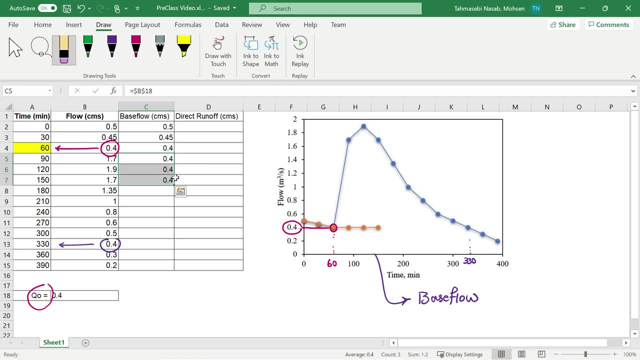 and then i'm going to move it all the way to next cell and next cell, and you can see that base flow is forming right over here as well, right, okay. and all the way to this point okay to, in other words, to this one over here, and after that point again, base flow is going to be equal to.